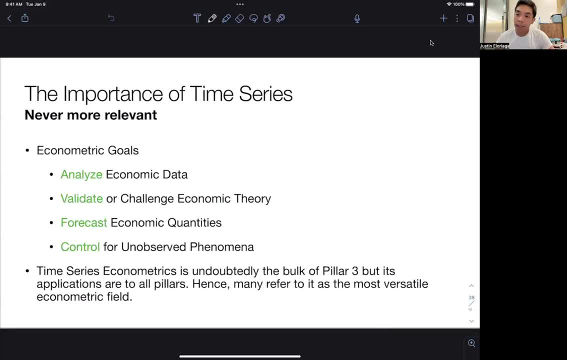 validate or challenge existing economic theory, forecast economic quantities and control for unobserved phenomena. And undoubtedly a bulk of pillar three, which is on forecasting economic theory, is to be able to analyze data, validate or challenge existing economic quantities. is related to time series, econometrics, primarily because we deal with 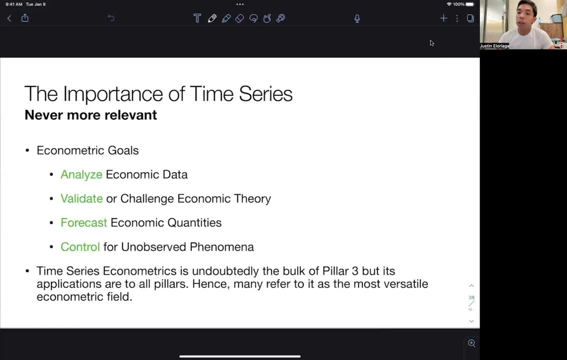 an abundance of data, which is time series, and economic quantities generally are time series variables, So it's a very versatile econometric field, one that has many applications, But in reality, what we denote as a time series, or understand as a time series, is not so simple. 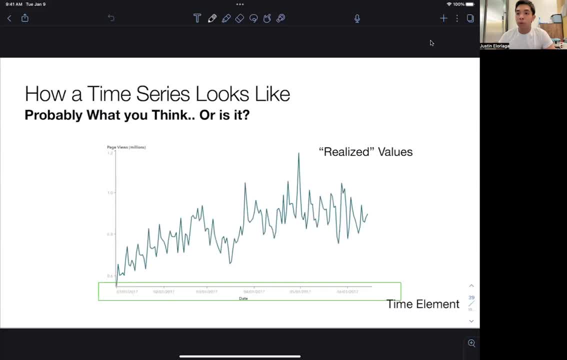 they say So. of course, if you sort of looked at any data set right, you would see there are tons of time series that exist in the world. There are many variables, many economic variables, non-economic variables that are time. 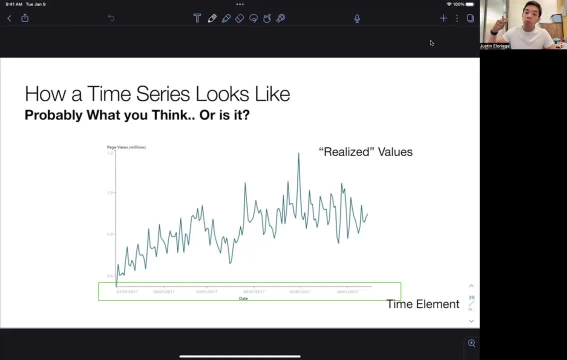 series variables And they're generally okay, realized values. When we say realized, it's what we observe right, Or what an agency or some person recorded as the actual thing that happened, right. So we have typically on the horizontal axis, when we plot a time series, data set. we have on the horizontal axis the date. 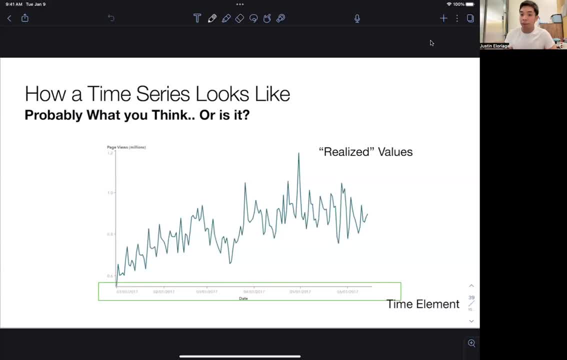 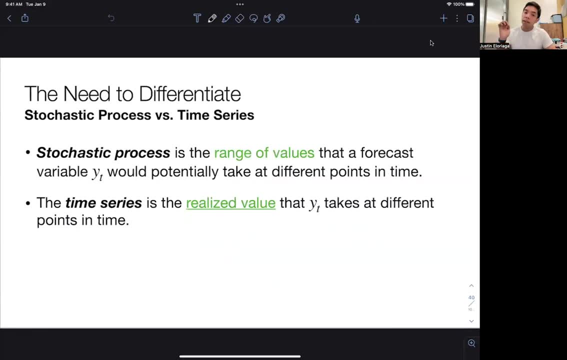 the date and you have on the vertical axis the value and then we plot it across time And generally that's what we perceive as a time series right. The key thing here is, in time series, econometrics. we care about both: the time series itself. 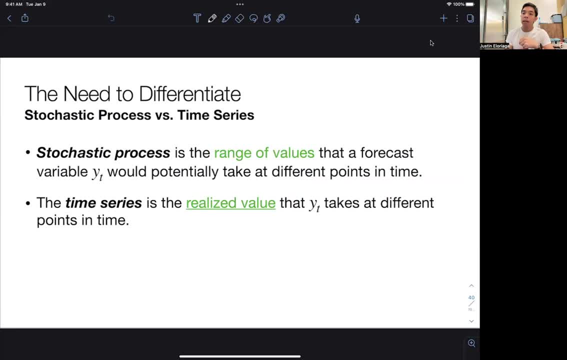 and something which we call the stochastic process. Okay, And in sort of building up our models, Okay, And in sort of building up our models, we actually consider more often than not the stochastic process first, right, So what is this stochastic process? Well, the stochastic process is the range of values that a forecast variable. 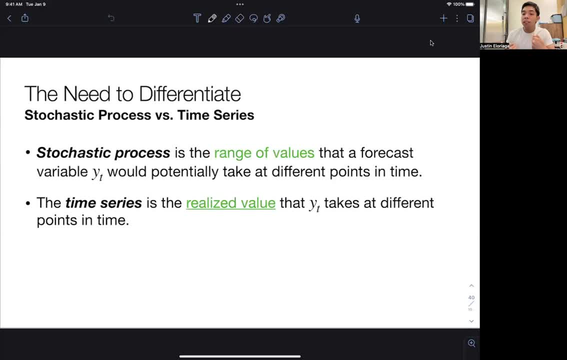 say Yt or any variable would potentially take at different points in time. Okay, The key thing here is: would potentially take and this range of values in general, right, it's sort of like a probability distribution. It's sort of like a probability distribution. It's sort of like a. 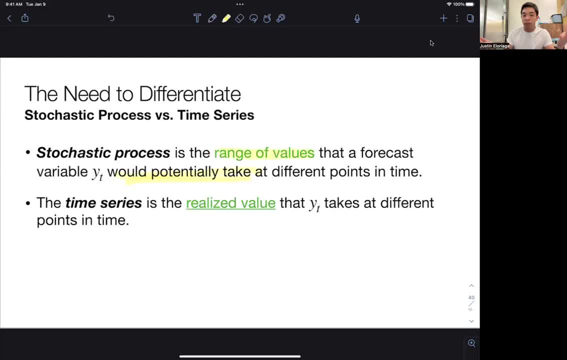 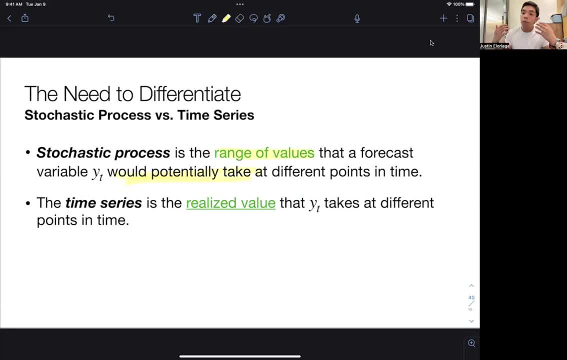 is generally a probability distribution of a particular variable at a point in time, And when we say it's a process, we collect all of those probability distributions across time, And that's what we refer to as the process. We'll see this later in the next few slides. Now, how does 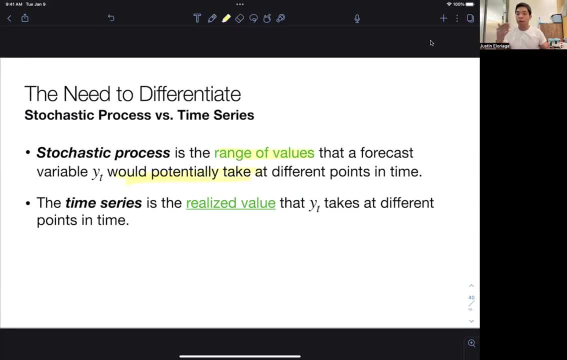 it differ from what a time series is. What do we really refer to as the time series? Well, a time series is effectively not a probability distribution. It's just a point, because it is the realized value that Yt takes at different points in time, So that time series exists. 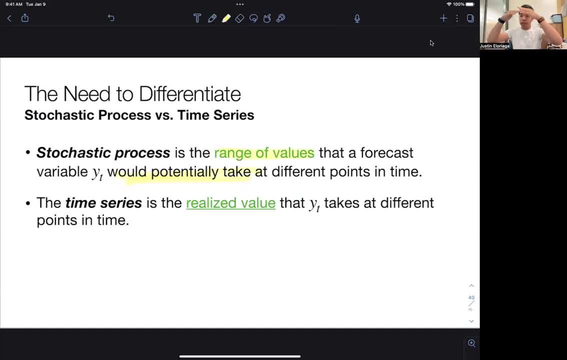 within the stochastic process, right, If the stochastic process is a probability distribution function, the time series itself is a point in that probability distribution function And it's the point that was defined in the probability distribution function And it's the point that was. 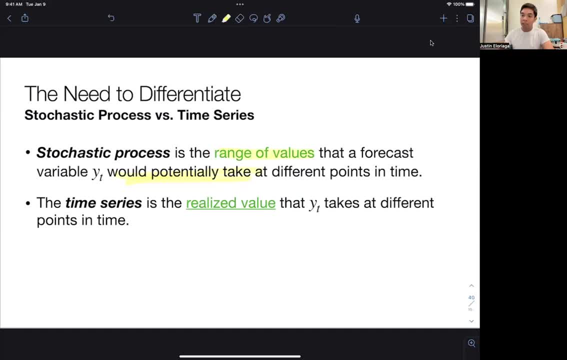 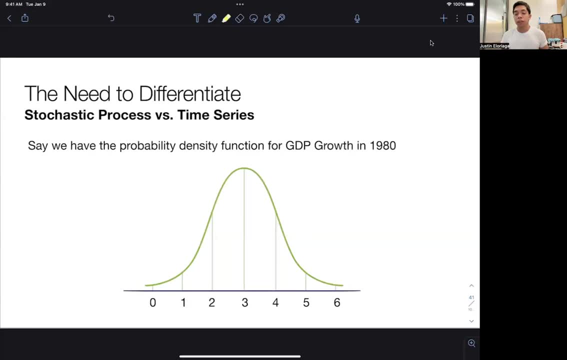 actually realized right, It's the realized value that Yt takes. So how do we sort of illustrate this? So say, we have a probability density function for GDP growth in 1980.. So of course GDP is generally a positive number but can take any. Of course we can have negative growth for 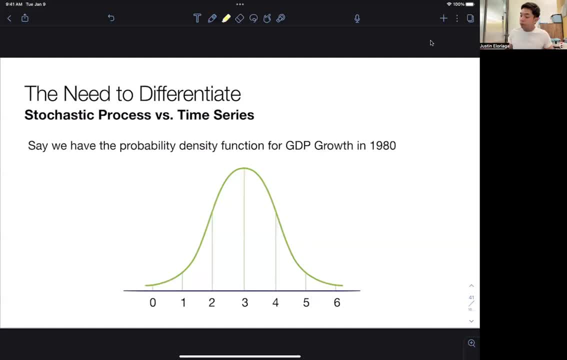 recessions, positive growth for expansions. And if you look at our example here on the average right majority of the mass okay is centered around 2% to 4% Okay. so for this country, the majority of the likelihood that their GDP growth in 1980 would be 2% to 4% is probably very high. The likelihood of a recession is very low. Also, the likelihood of a very big sharp growth above 6% is very low. So majority of the mass okay of this GDP growth in a particular point in time is centered at 2% to 4%. 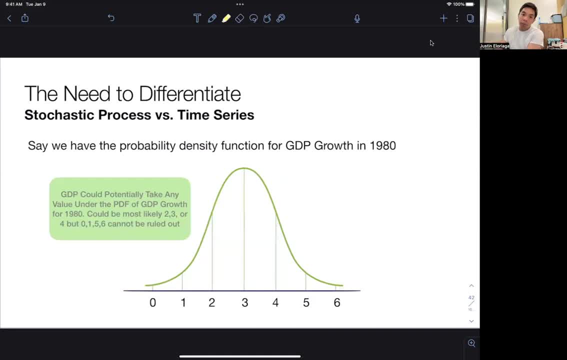 Okay, Now the GDP value could potentially take any value under the PDF, right? So whatever realized value that could be in 1980 could be within this PDF. But again, it's most likely two or three. but you can't really rule out the edges, right, Because it's a random thing, right. 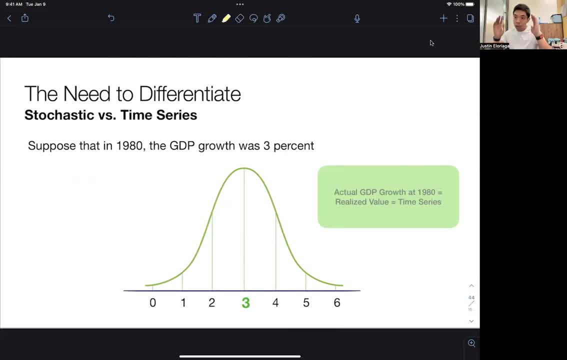 So suppose now, okay, that the GDP growth in 1980, when it actually happened, was 3%, Okay, that 3%. so if say, say 1980, okay, and GDP grew by 3%, that point starts basically the time series. 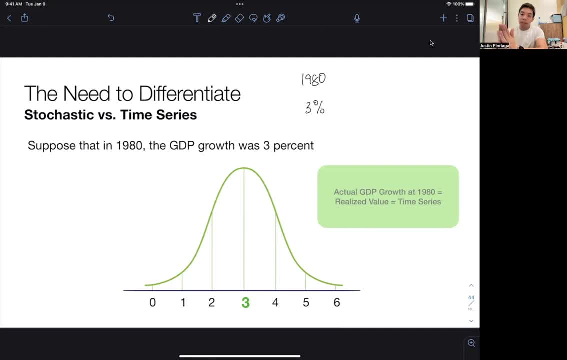 because that was the realized value. That was what actually happened in 1980. It is the start of our time series. It's the start of the realized value of the series. Okay, And if you want to understand the stochastic process, quite simply think of it as this: Say: we have here four years. 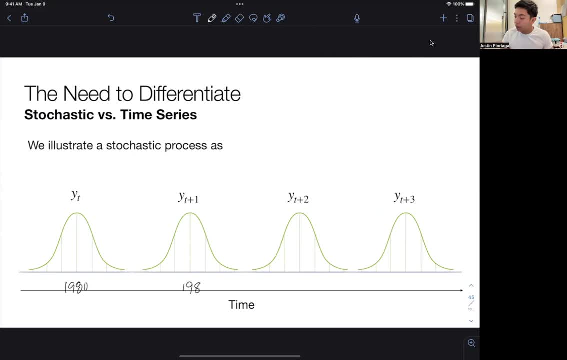 say we have 1980, 1981, 1982, 1983.. A stochastic process is generally a collection of different probability distribution functions across time that pertain to a particular process. So in here say this is GDP. okay, we have a stochastic process here of GDP from 1980 to 1983.. We see the 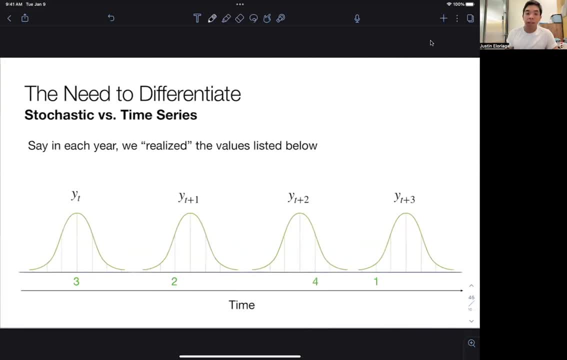 different PDFs for each of these years. right, Okay, Okay. And for example, in 1980, we have 3%, as the realized. In 1981, we have 2%. 1982, we have 4%. 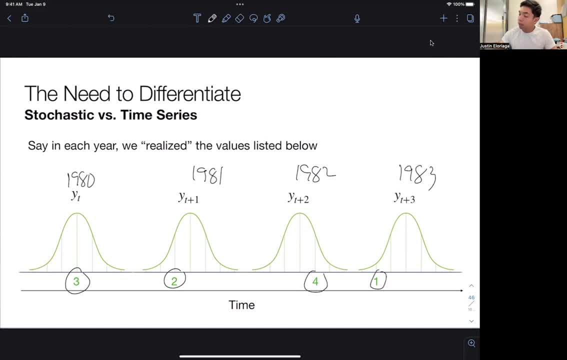 1983, we have 1%. So the time series is going to be 3%, 2%, 4%, 1%, right. So, if we plot this right, if this is 1980, 1981, 1982, 1983, okay, 1,, 2,, 3, 4.. In 1980, it was 3%, right. 1981, it was 2%. Then we have 4%. 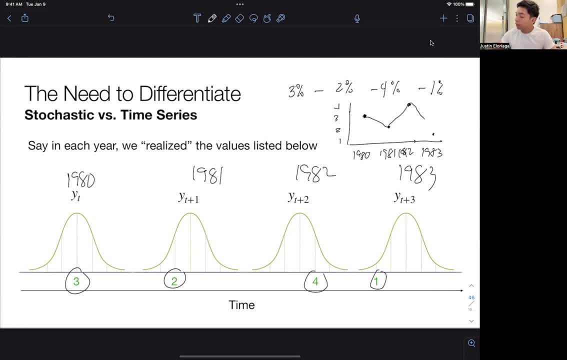 Then we have 1%. So if we plot it, this is our time series. It's the realized value of what went on in that year. The stochastic process is basically the collection of the PDFs across the years. Okay, So that's the difference between a time series and a stochastic process, right? 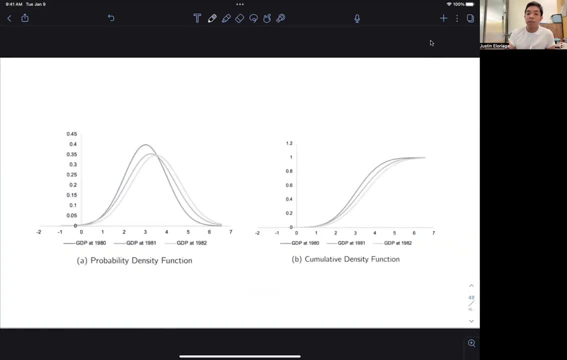 So the collection of all these realized values is the time series. The collection of the PDFs is the stochastic process. You can even illustrate it further. right, You can overlay these PDFs into one graph, as I did here in graph A, And because this is a PDF, it has a corresponding cumulative. 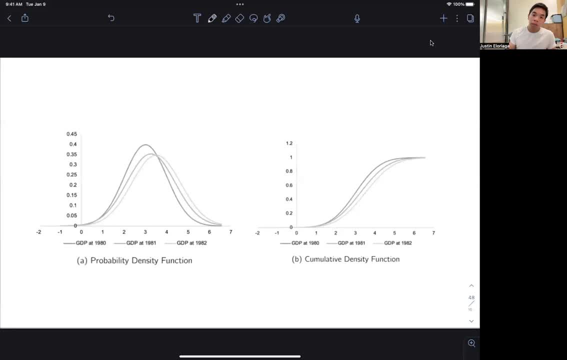 density function, or CDF, which sums up to 1.. So that's how we view the, the stochastic process. So that's it for this particular video. In the next video we'll deal with stationarity. So thank you for your attention and I'll see you in the next video. Thank you very. much.